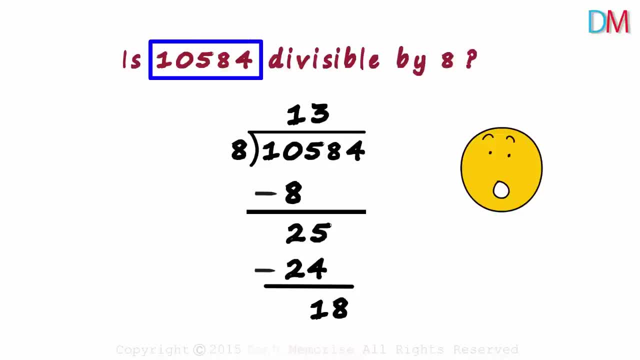 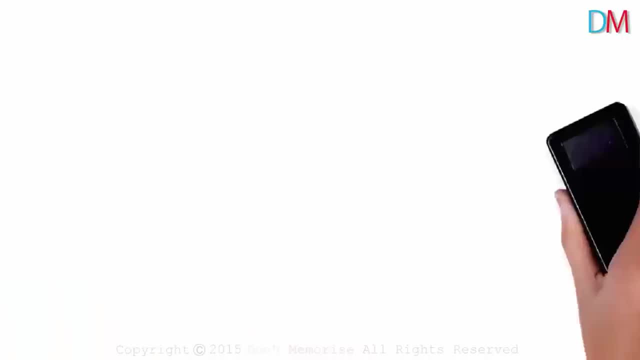 These rules will help us know if a big number is divisible by another number, And yes, within 5 seconds. Before we move on to the shortcuts, we need to know something about the number zero. Any number multiplied by zero results in a zero. 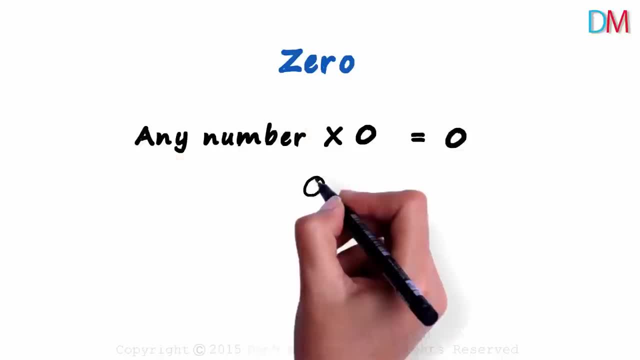 Transposing any number to the other side, we can say that zero divided by any number will result in a zero. What does this tell us? It tells us that the number zero is divisible by any non-zero. It tells us that the number zero is divisible by any non-zero. 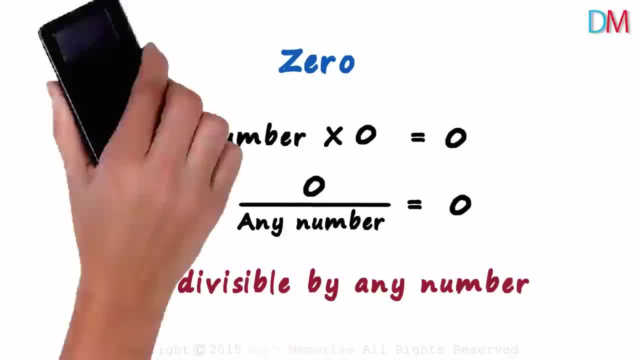 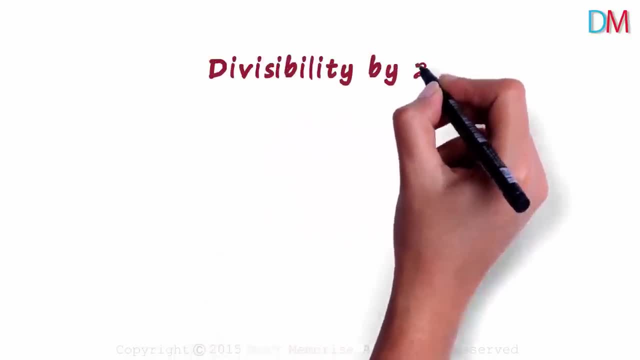 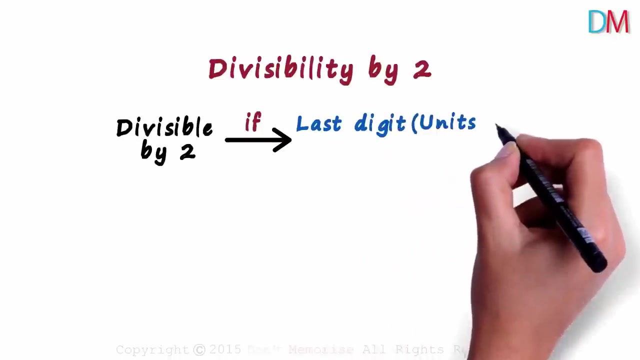 First let's look at divisibility by 2.. How can you tell if a number is divisible by 2 without performing any division? Here's the simple rule. Well, a number is divisible by 2 if the last digit, that is the units digit of that number. 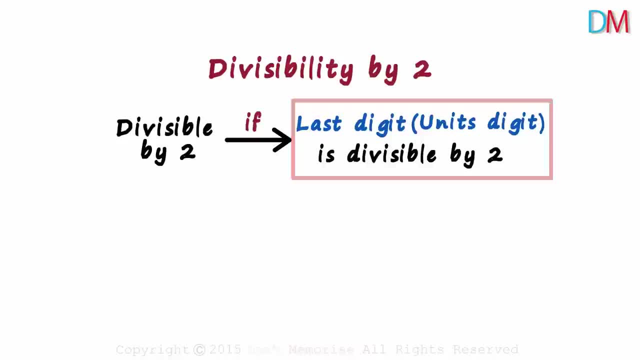 is divisible by 2.. What does that mean? Let's look at a couple of examples to see how easy it is to know. Here's the simple rule. Let's look at how easy it is to know. What does that mean? Here's the simple rule. 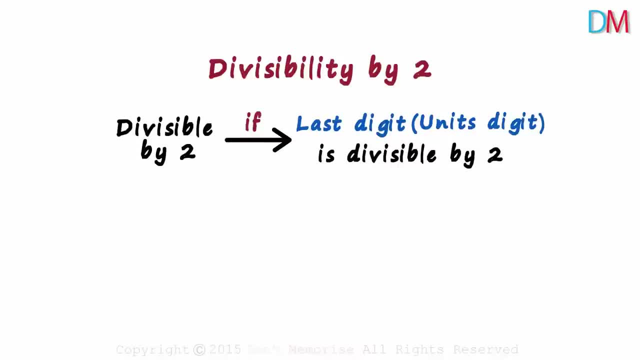 Let's look at how easy it is to find out if the number is divisible by 2.. Here's your first number: 982,356.. Is this number divisible by 2?? To answer this quickly, we just need to look at the last digit. 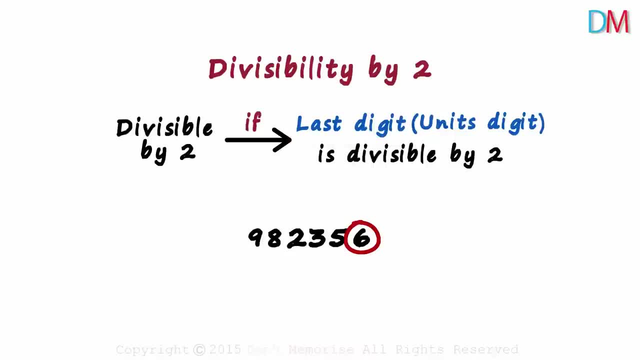 To answer this quickly, we just need to look at the last digit. The last digit is 6, and since 6 is divisible by 2,, the entire number is divisible by 2.. 982,356 is divisible by 2.. 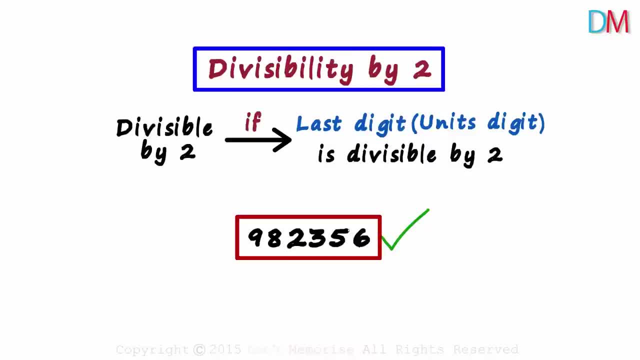 982,356 is divisible by 2.. Let's hoping that's easy enough and it's clear. Our first immediately step is to learn two points which will guide you to find out divisible by 2.. Here's the second number: 10,987,659. is this number divisible by 2?? 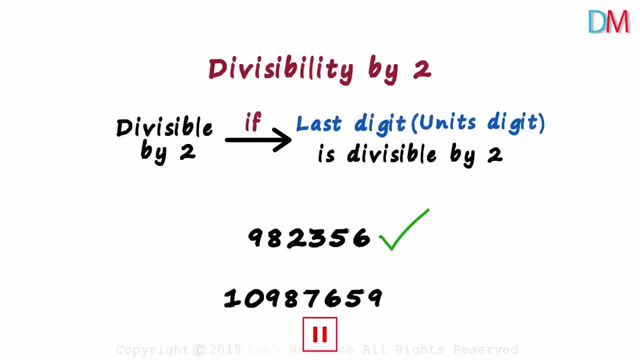 Pause the video and try it out. Is this number divisible by 2?? The units digit of this number is 9.. Is 9 divisible by 2?? No, And that is why this number is also not divisible by 2.. That's how. 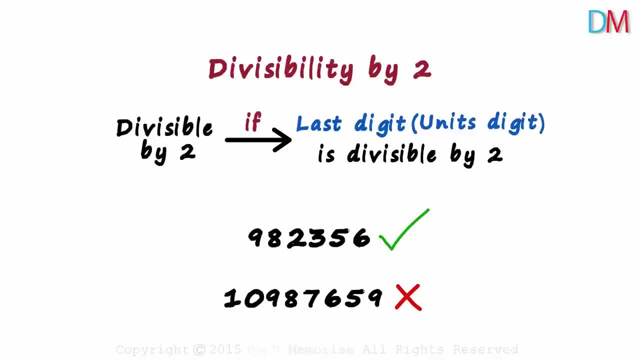 simple it gets with divisibility rules. Imagine how much time it would have taken you to manually divide these two numbers by 2 and see if the remainders are 0 or not. Now let's move on to the second rule: Divisibility by 4.. How can we? 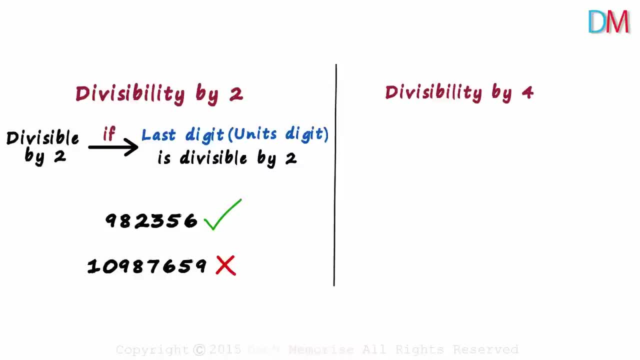 quickly tell if a number is divisible by 4?? It is pretty similar to the divisibility table Divisibility test of 2.. A number is divisible by 4 if the number formed by the last two digits is divisible by 4.. In this case it is the last two digits. In the case of divisibility, 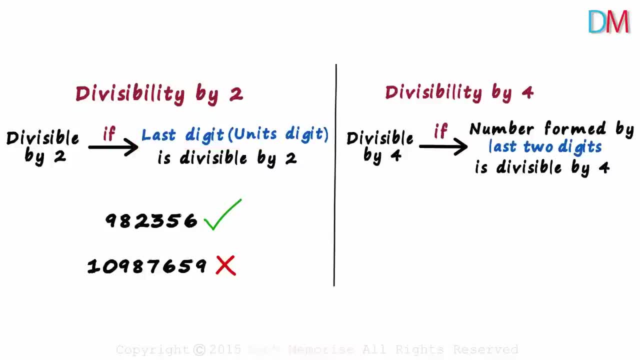 test of 2,. we just had to look at the last digit. So is 1,987,632 divisible by 4?? As it's divisibility by 4, we need to look at the last two digits. The number formed by the last two digits is 32.. Is 32 divisible by 4?? Yes, So this? 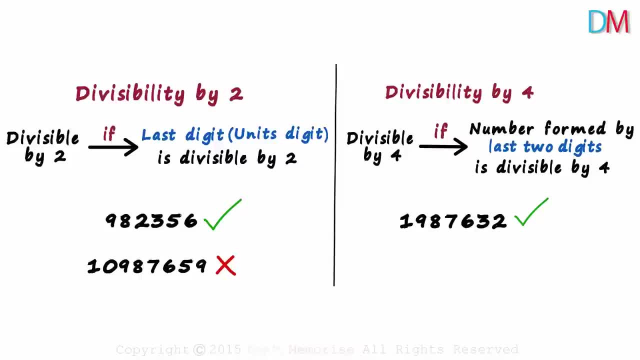 big number is also divisible by 4.. Here's the next one. Is 97,432,100 divisible by 4?? What are the last two digits here? 0 and 0. The number formed by the last two digits is 0. And we learnt that 0 is divisible by 4.. 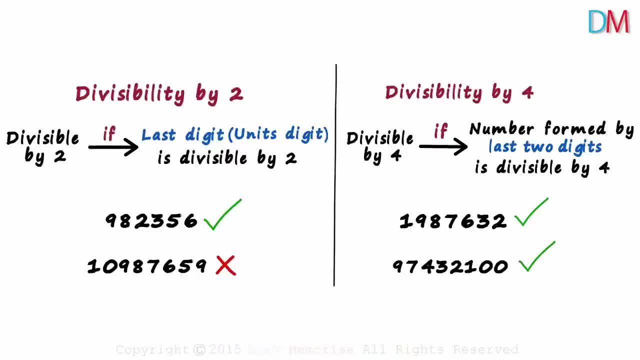 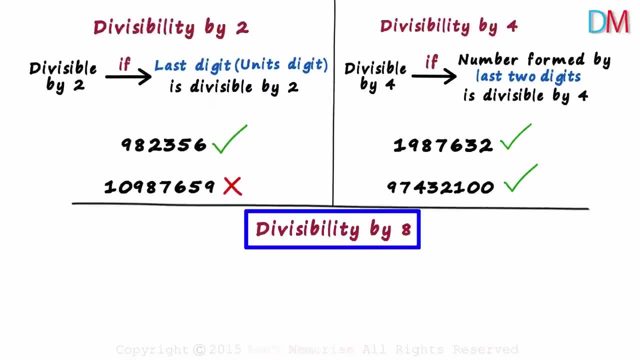 any number. Hence this number is also divisible by 4.. And now we come to the last divisibility rule of this session, DIVISIBILITY BY 8. A number is divisible by 8 if the numbers formed by the last 3 digits is divisible. 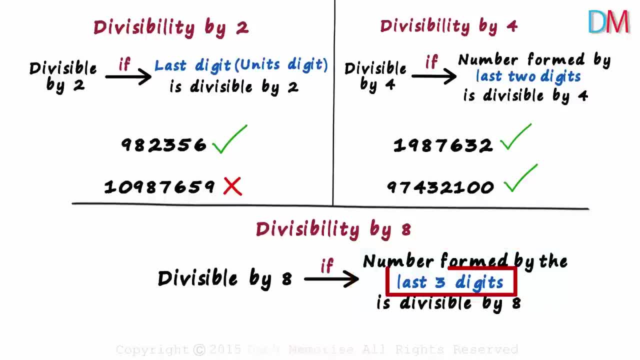 by 8.. Yes, numbers formed by the last 3 digits. Look at the number 16,998,048.. Is it divisible by 8?? The last 3 digits are 048.. The number formed by the last 3 digits is 48.. 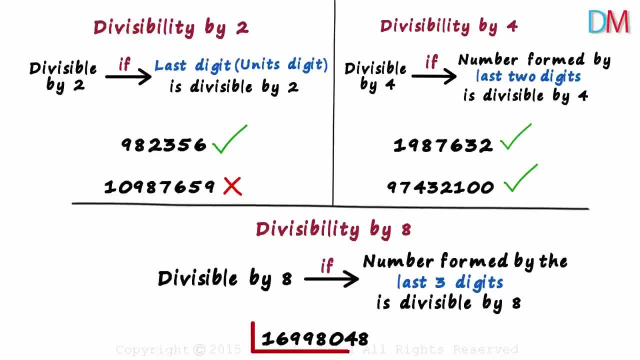 And 48 is divisible by 8.. So this huge number will also be divisible by 8.. Wasn't the rule simple? For a number to be exactly divisible by 2, its last digit should be divisible by 2.. To be exactly divisible by 4, the number formed